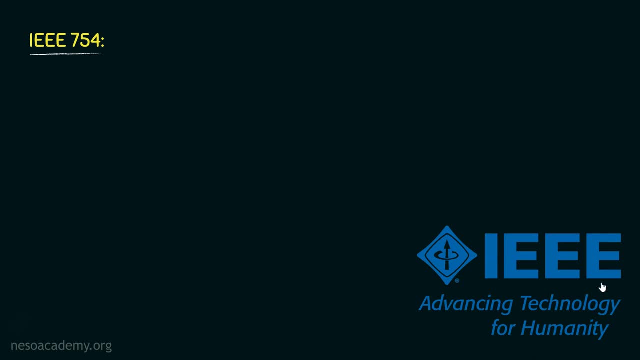 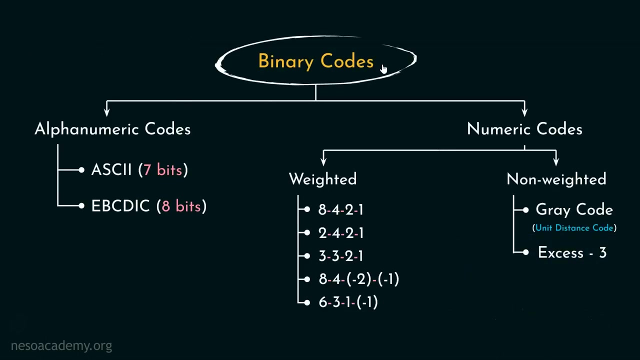 the Institute of Electrical and Electronics Engineers comes at rescue. Basically, they have specified the particular standard 754 for representation of the floating point numbers. Now, honestly, this is not new to us. If you remember, while we studied about the binary codes, we came across the ASCII and the EBCDIC codes. 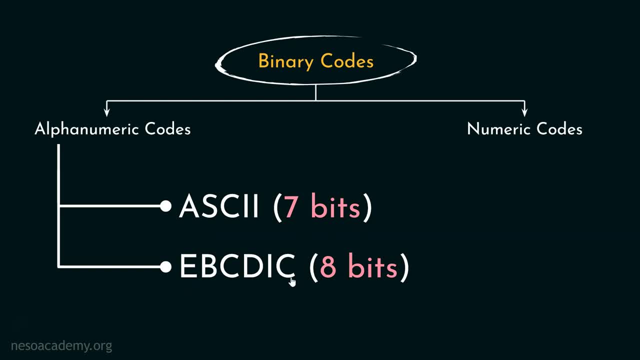 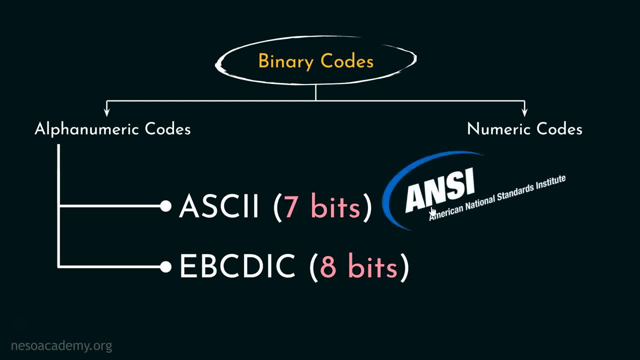 Coming to ASCII. the 7 bits of ASCII were specified by ANSI. Now, coming to EBCDIC, the specification that these will also be of 8 bits was made by IBM. Basically, what I'm trying to say is that whenever some standards are specified, 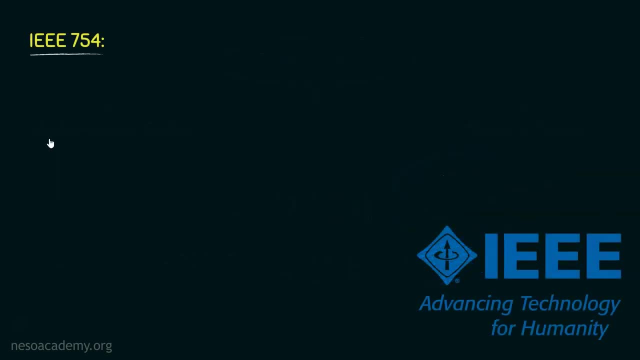 there must be some organizations behind it, and the IEEE is responsible for the standardization of the floating point numbers, numbers Now, IEEE 754 is actually a technical standard for floating point arithmetic, established in 1985 by the Institute of Electrical and Electronics Engineers. Now, honestly, I don't. 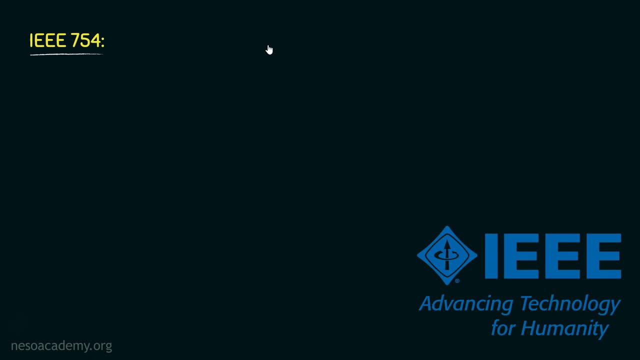 really want to bore you with all these historical details. Nonetheless, I do want to mention the milestones in this particular regard. So the first standard of IEEE 754 was developed in 1985 and it was named as IEEE 754-1985.. Now these particular standards were revised in the year. 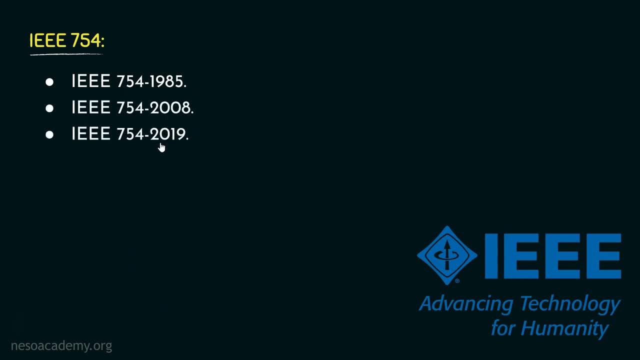 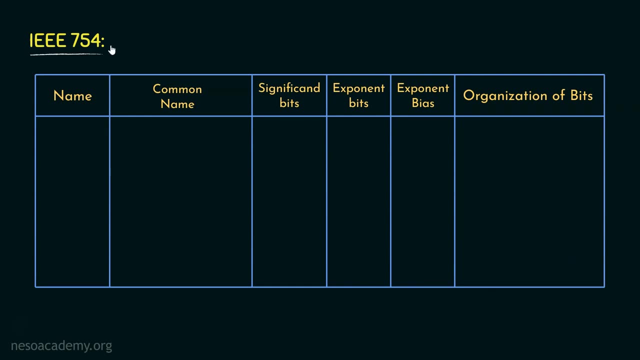 of 2008 and the latest revision was done in the year 2019.. Now, over this time period, IEEE 754 actually defined quite a lot of standards, So we will get to know about them, one after the another. So the first one is binary 16.. Here the 16 stands for the number of bits specified for this. 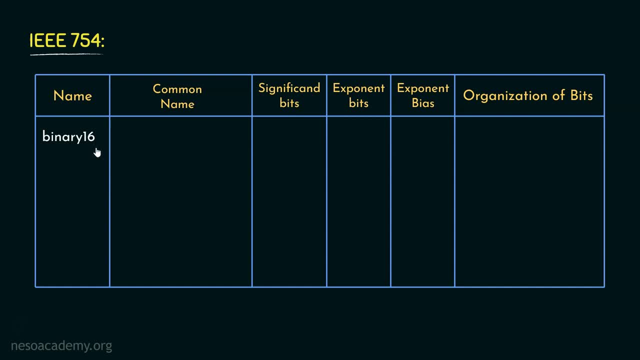 particular standard, Now binary 16, this standard is commonly known as half-precision. Now, here for significant bits, we have 11 bits. Now what are significant bits? This is actually the accumulation of the sign bit and the mentissa portion, which, in case of binary 16 or half-precision, is 11.. Now think about it. 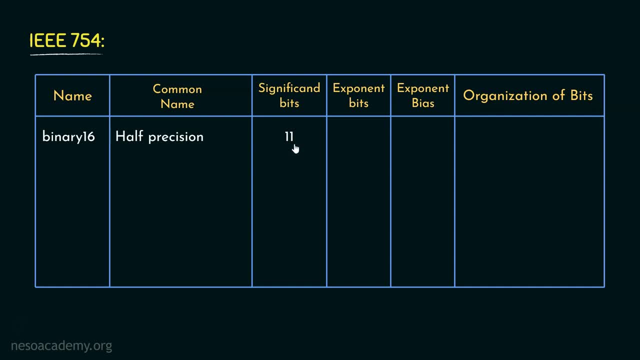 If 11 bits are specified for the sign and the mentissa portion, how many bits will be specified for the exponent bits? It is going to be 5, because in total we have 11 bits. Now, how many bits will be specified for the exponent bits? It is going to be 5. 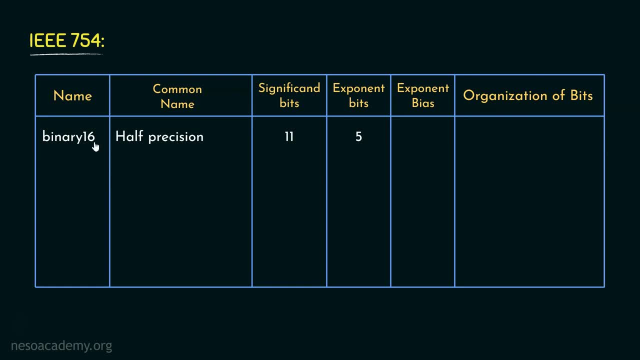 because in total we have 16 bits. Isn't it Now for binary 16 or half-precision? we have the exponent bias as 15.. And finally, the organization of bits is something like this: That is the MSB, is the sign. 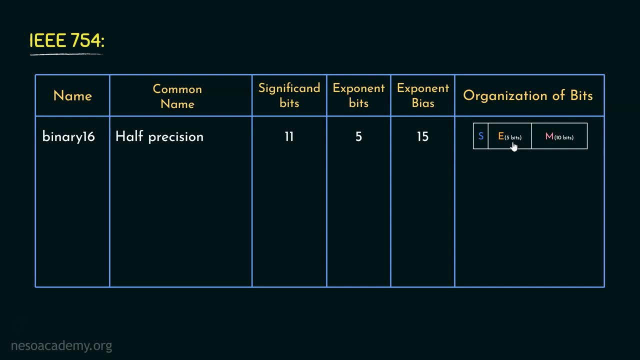 bit. Thereafter 5 bits are specified for the biased exponent And finally, the remaining 10 bits are used for the mentissa portion. Now let me illustrate how the biased exponent works in case of IEEE 754 standards. As you can see here for exponent bits we have the exponent bias as 15.. 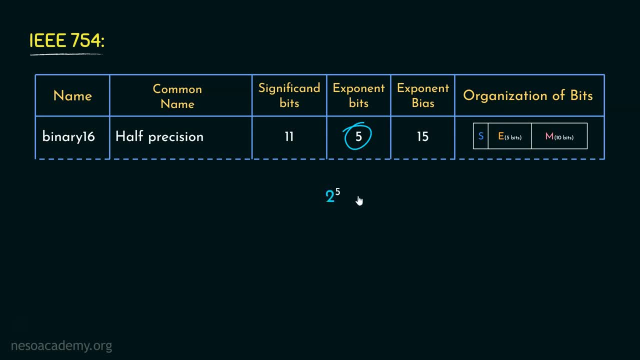 For exponent we have 5 bits, So using this we will obtain 2 raised to the power 5, that is 32 pattern Right Now. considering unsigned numbers, this will be 0 to 31.. Basically, this is the range. 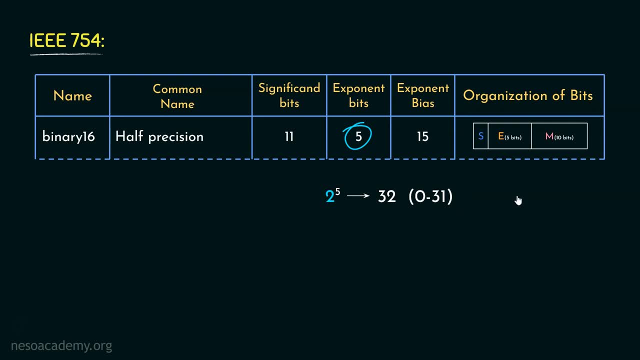 in terms of unsigned numbers. Now, if we are going to use 2's complement, in that case the range of values that we could have obtained using 5 bits is going to be minus 16 to plus 15.. Correct, Where the pattern for 0,. that is all 0,. 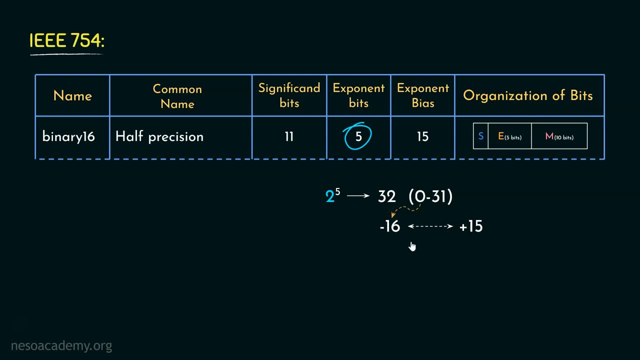 would have represented the exponent minus 16.. And, on the other hand, the pattern for 31,, that is, all 1's, would have represented the positive exponent plus 15.. However, this particular range is not followed in case of IEEE 754 standards. Instead, the range which 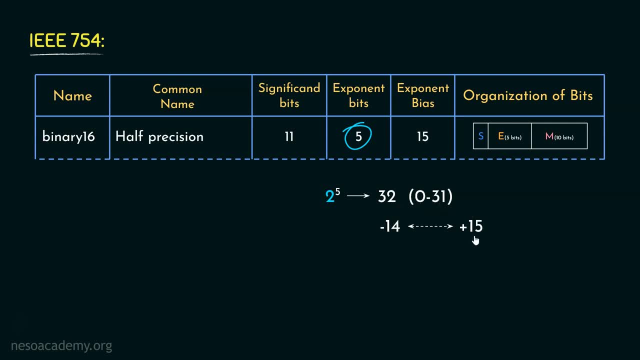 is covered by the exponent bias is from minus 14 to plus 15.. And the reason behind that is the first pattern, that is all 0's, and the last pattern, that is all 1's. these two patterns are used to represent something else which we will get to learn about in the next session. 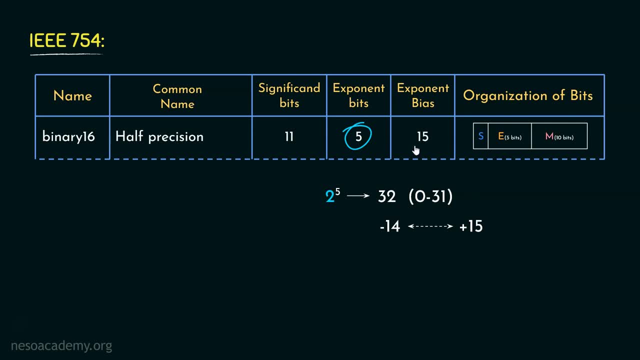 Anyway, for now, just remember this: if the exponent bias is 15,, then the minimum exponent is going to be minus 14,, that is, 1 less than this value, and the maximum exponent will be positive 15,. that is this value only. So this is how, in case of IEEE 754 standards, 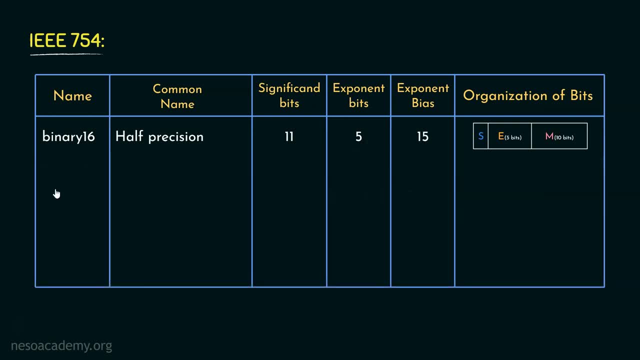 the biased exponent works. Now coming to the next one. it is binary 32, which is commonly known as single precision, And this one specifies 24 bits for significant bits. And since 24 bits are combinedly representing the sign and mantissa, therefore 32 minus 24,, that is, 8 bits, will be used for exponent. 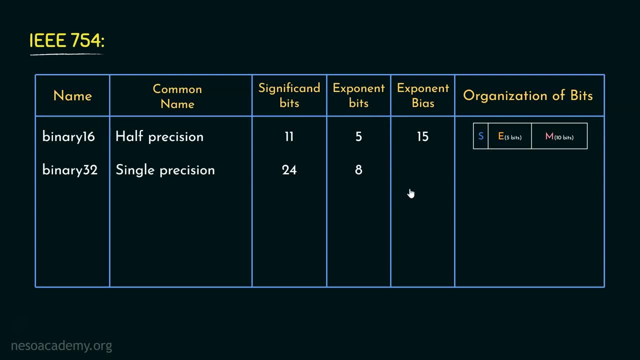 And since 8 bits are being used for exponent, the exponent bias is going to be 127.. Therefore, coming to the organization of bits, it is going to be something like this: the MSB will dedicate the sign bit Thereafter. next, 8 bits will be for the biased exponent. 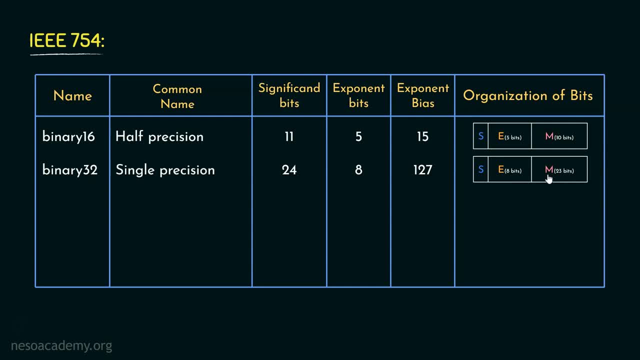 and finally, 23 bits will be specified for the mantissa portion. Coming to the next one, it is called binary 64, which is commonly known as double precision, where 53 bits are specified for the significant and 11 bits are used for exponent, which also. 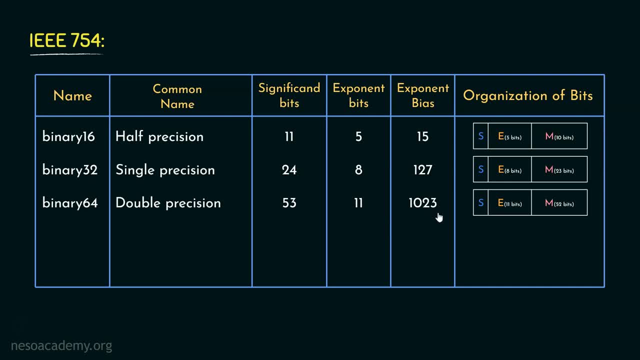 has the exponent bias of 1023.. And the organization of bits are something like this, where you can see the MSB is again dedicated for the sign bit and thereafter 11 bits are used for exponent And finally, the remaining 52 bits are being used to represent the mantissa portion. 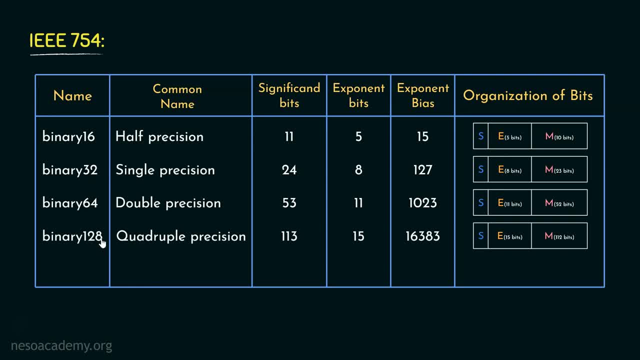 Now coming to the next standard. it is called binary 128.. Basically, 128 bits are used in this particular standard, which is commonly known as quadruple precision, which specifies 113 bits for significant and 15 bits for exponent having the exponent bias as 16383. 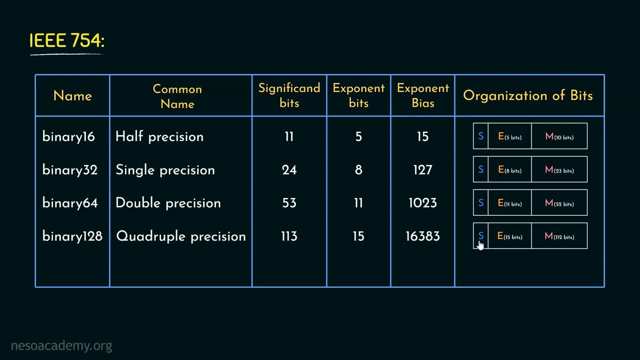 Now, coming to the organization of the bits. observe here also the sign bit is specified by the MSB. Thereafter, 15 bits are dedicated for the exponent and finally, 112 bits are dedicated for the mantissa. Finally, the last one is known as binary 256, and from the name only we get to know that. 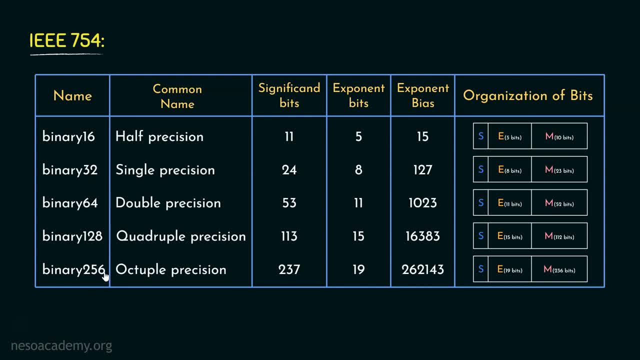 256 bits will be dedicated in this particular standard, which is commonly known as octuple precision, and from this 256 bits, 237 bits are used for the significant. remaining 19 bits are used for the exponent leading towards the exponent bias.